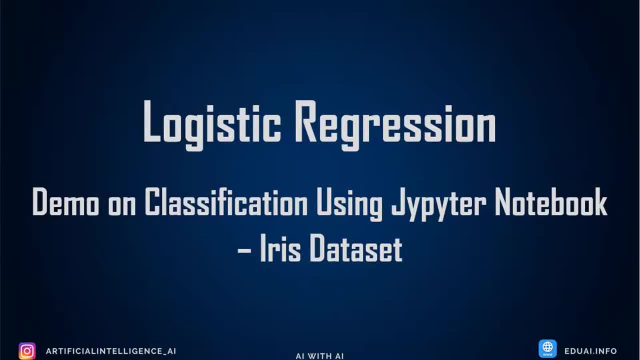 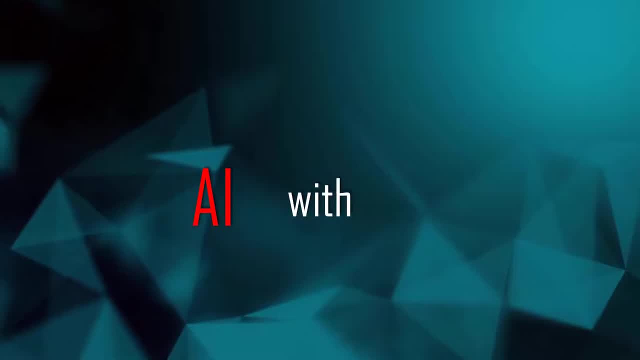 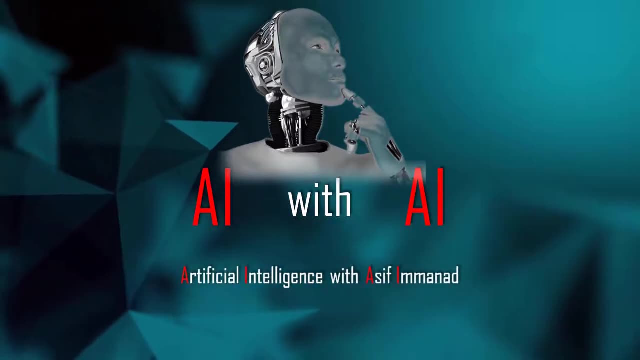 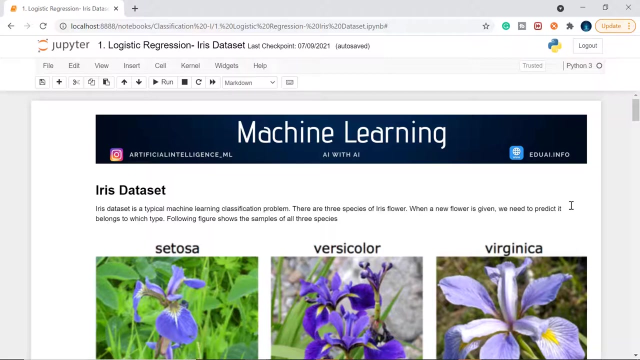 Hey guys, welcome to AI. with AI once again This side, Asif Himnad. Now let's see a demo on the classification, as I promised, In the last videos we have seen what is machine learning and what are the different types of machine learning, and the recent video we have also discussed about the classification and the different examples. 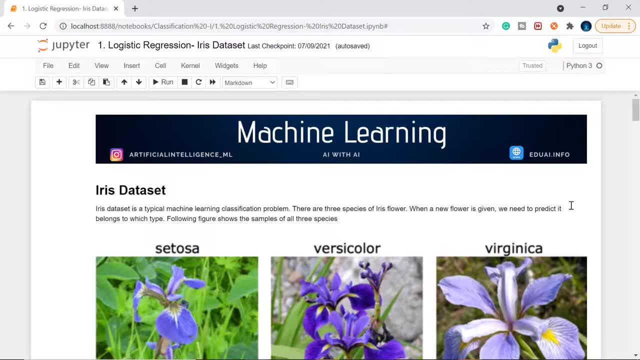 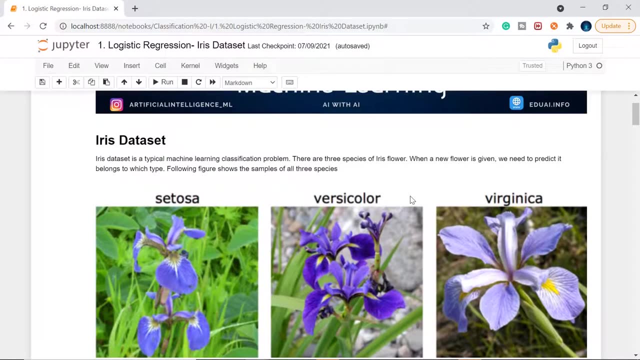 And we will be starting with the very small and simple example so that you guys can also implement. Okay, so this is all about IRIS dataset and the classification and it's a typical machine learning classification problem, right? So what we need to do here? there are three species of the flower, that is, Cetosa Versicolor and Virginica. 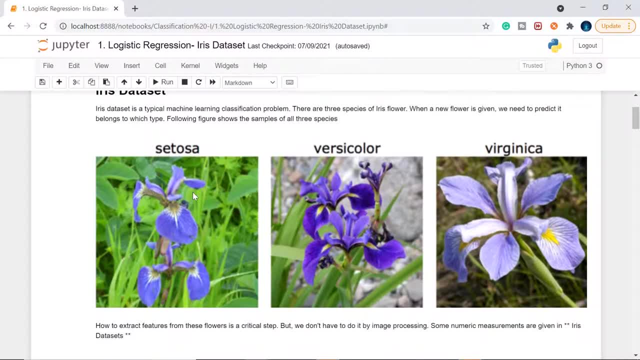 That's an IRIS flower right. So we need to predict, given three species of the flowers to the model, train that model on given data, And then we need to predict the species of the flowers to the model And then we need to predict the species of the flowers to the model. 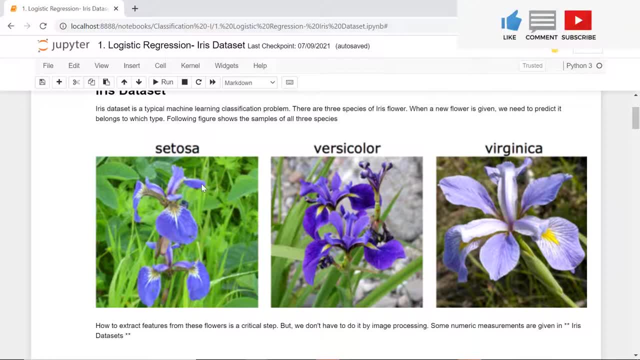 And, when any new flower is given, find out which type that new flower falls into, whether it is Cetosa, Versicolor and Virginica. Definitely we won't be having photos here. That's part of image recognition and feature extraction. 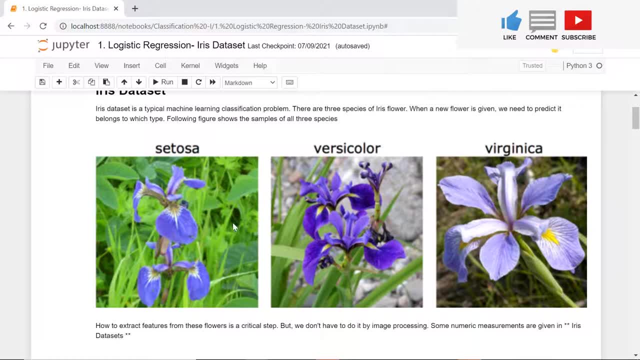 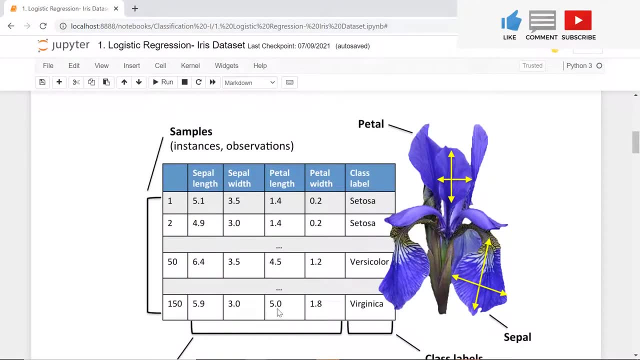 That's a part of deep learning. We'll see that later in the deep learning series, But for now let's focus only on the machine learning part. right? How do I get the data here? So we have a data in the table. okay, in the numerical form. 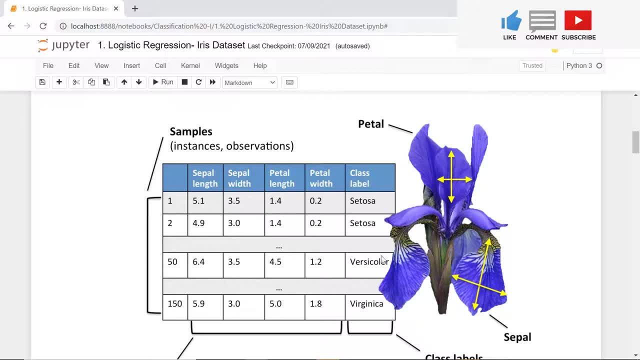 Definitely. even if you extract the features in a computer vision, When the image extraction happens, it actually looks at the features and puts them into the numbers. Okay, this is what we are doing manually here For now. we don't have the image extraction for now. right? 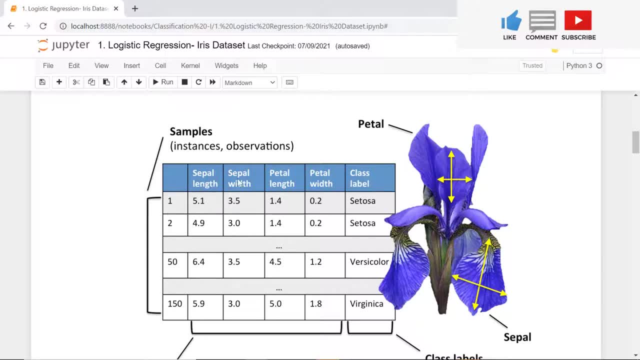 So we have a data in the table where we have sepal length, sepal width, petal length, petal width and the class label as the column. What do you mean by the sepal length? So the lower part of the flower is called sepal. 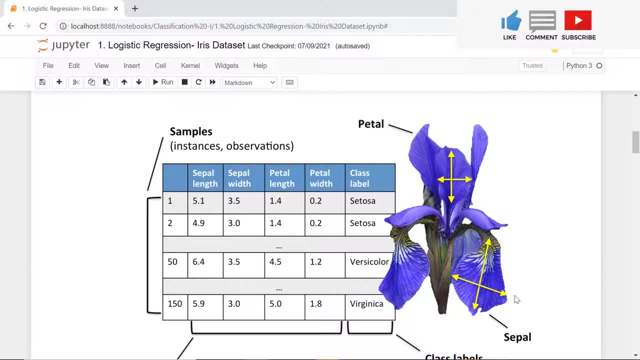 So we have sepal length and the sepal width given And we also have the upper part, which is called sepal length, Which is called the petal right. So this is petal length and petal width is given. So if the sizes of the flowers- petal and sepal length, the measurements are given, based on that, the prior data is given. 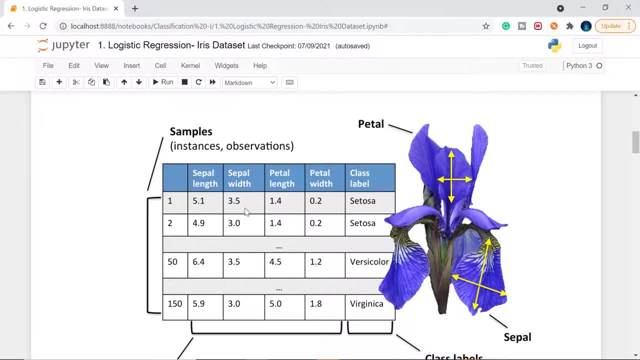 So if it is sepal length is 5.1, sepal width is 3.5, petal length is this and petal width is this, Then this flower is a setosa. So this data is given. So this is supervised learning right. 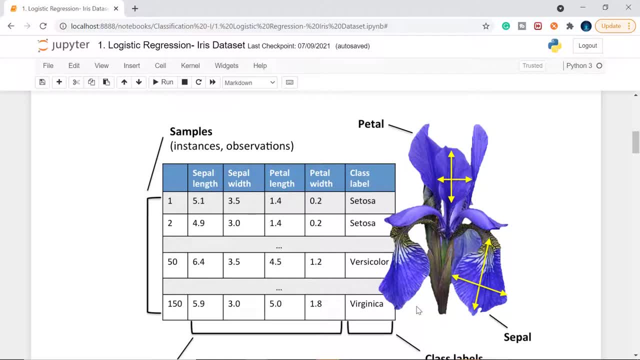 So the measurements, that is, X column, X values And the Y values, that is, output- is also given. So we have a correct data already in supervised learning. Right answers are given already. We need to find more right ones. So in future, when I receive new flower measurements, I need to find out which. 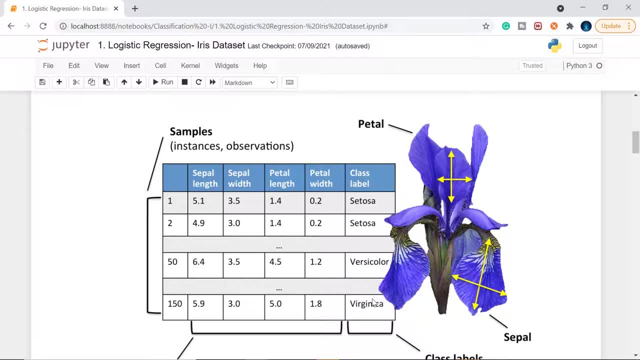 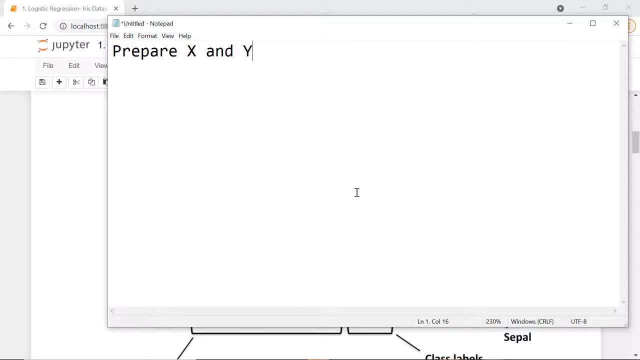 class it belongs to: setosa, versicolor or virginica. Simple. So what steps we are going to follow? Let me quickly tell you the steps. It's very simple, right? We have already seen this. Prepare X and Y. X is your input. 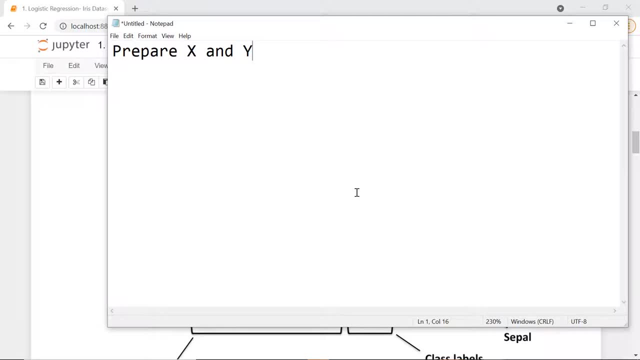 Y, is your output Supervised learning right? We have right answers given. You need to find more right ones, And once you prepare X and Y, next step is to choose which algorithm you want to use, That is, import machine learning algorithm. 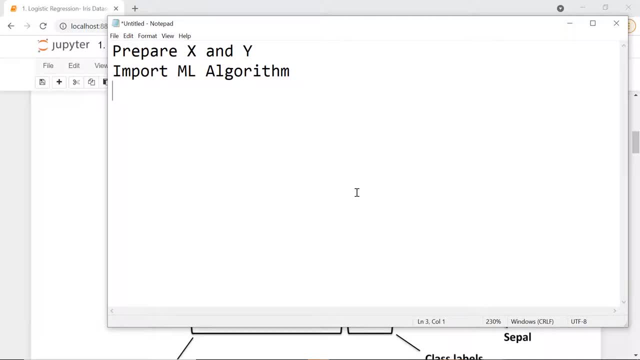 OK, so once you choose which algorithm you want to use, you will train the machine learning model on the input Right. So you will be training the machine learning model Right And this is called. we have a simple method. If you remember, that is called model dot fit. 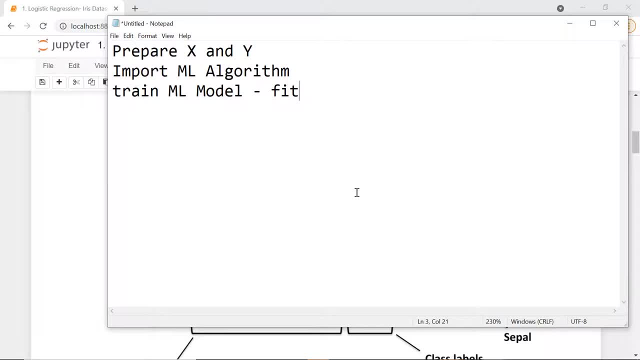 Right, If you visualize your algorithm, then you'll be training this. That is model dot fit. Once the machine learning model is trained now your model is ready to predict based on the new input given. OK, so these are the simple four steps that we guys are following in machine. 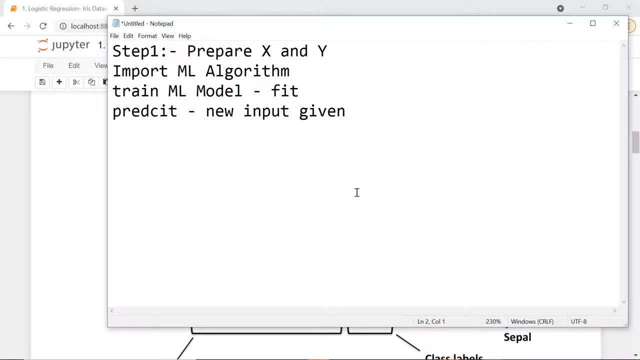 learning, so that we can easily see the demos, easily see the examples on it. Right? So this is super easy. OK, so these are the four steps that we follow, Right? Other than this, we are going to also see a model dot score. so, 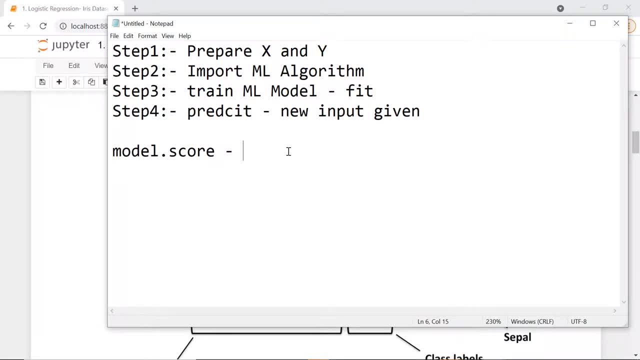 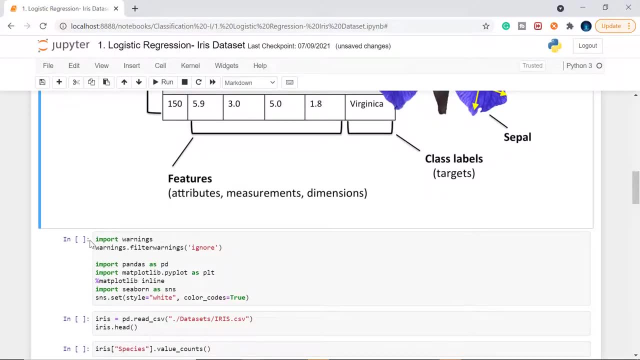 we can check what is the accuracy of my model, whether it is 90 percent, 90 to 95, whatever. OK, so let's jump on the demo. Please focus only on the cells which I'm executing. OK, so this is the first cell that I want to execute. 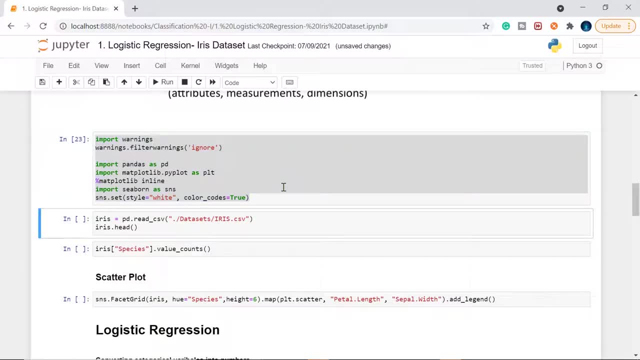 I use shift enter to execute this cells. OK, so what we are doing here? ignoring warnings, importing Panda, Matplotlib and Seaborn? OK, so these are the three data science libraries which are required to plot the data to find out the insights. 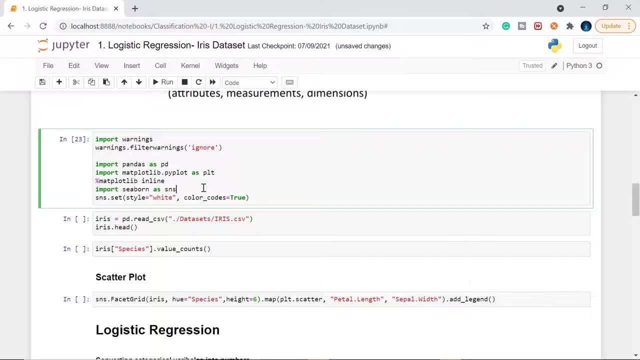 of the data so that I can understand what type of, what is the nature of the data. Right Based on that, I can take the decision which algorithm I should use. which algorithm is the best fit? OK, we have discussed this already, so I don't waste my time here. 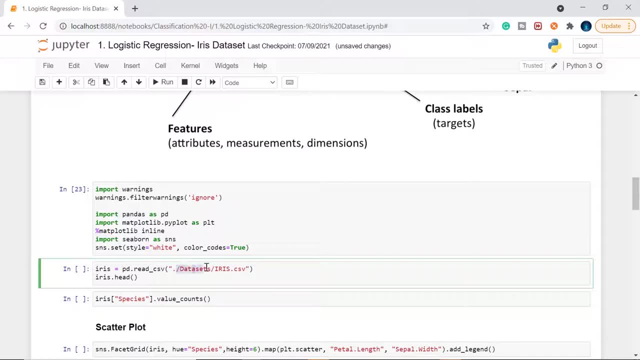 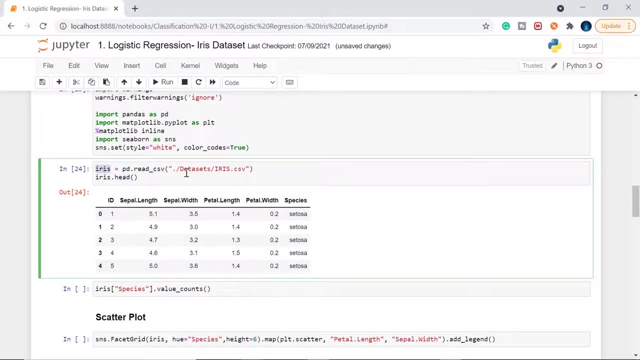 This data is already. we have in the CSV format, Right, I kept it in some directory. I'm reading that data, So this is how the data looks like And I restarted. So this is Iris is our data And I'm reading only the head. 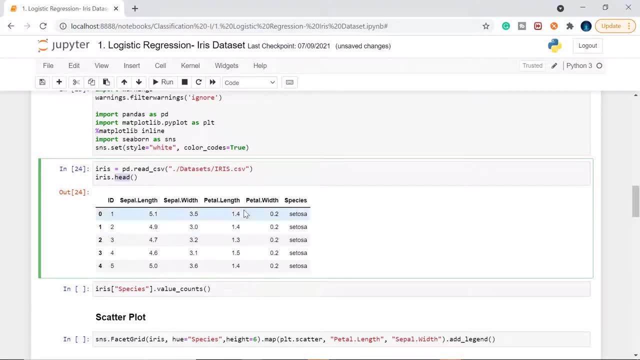 That means first five rows Right, So you can see sepal length, sepal width, petal length, petal width and the class of that flower going ahead. So what I did here, I have got data frame Right. If you don't know about basic data science, 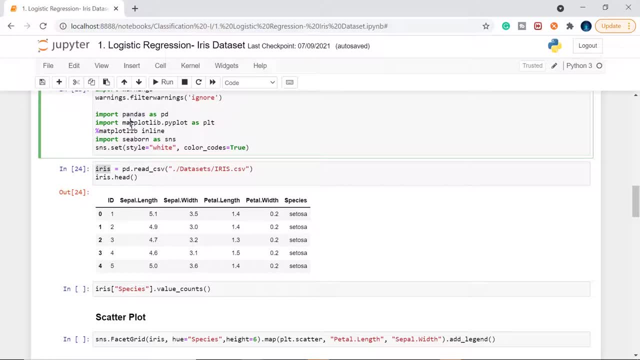 Python libraries I urge you to understand Pandas, Matplotlib, Seaborn, NumPy. So these are four basic Python libraries that everyone must understand. Right Iris variable is a data frame here, so that I can perform operations on the table. 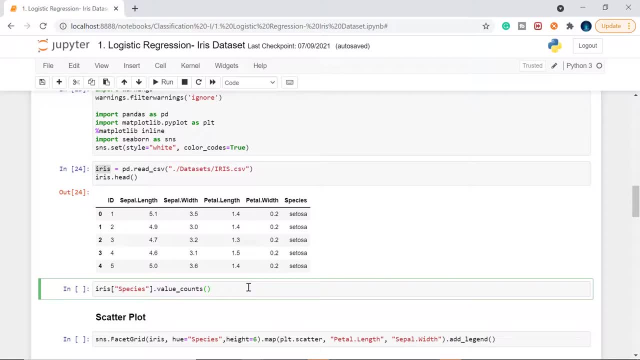 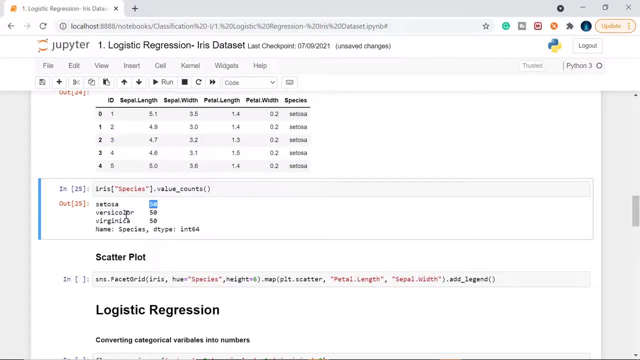 OK, now, once I have the data frame, let's see what are the total counts I have. I mean, how many different types of flowers I have. I have 50 setosa, 50 versicolor and 50 virginic. I mean we have 150 rows here and all are of type integer. 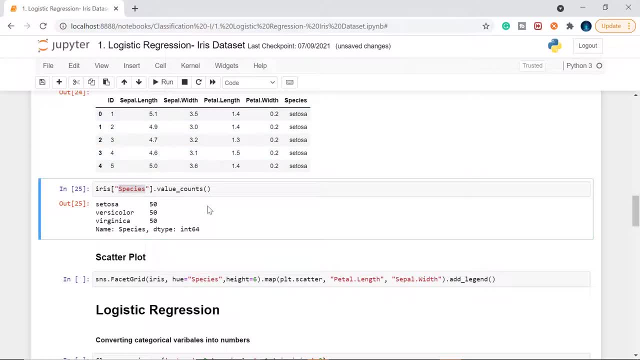 And we are doing the count on the species only. OK, so I just wanted to understand if the data is not biased. Yes, And data is not biased. We have 50, 50 each. So let's train our model and use logistic regression here. 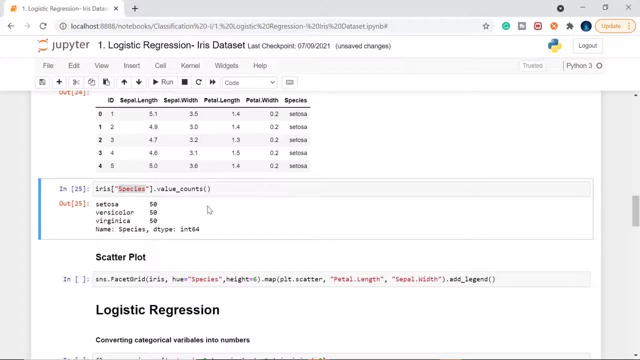 Yeah, But before doing that, you know, I just want to see how does my data looks like, because there are three types, There are three classes, Right, And how do they look like? So, to see how does the data look like, I'm using a scatterplot here. 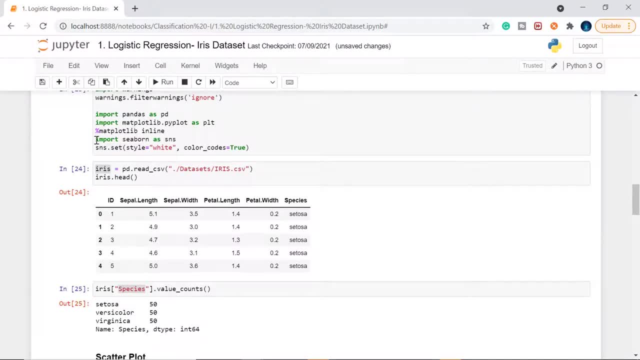 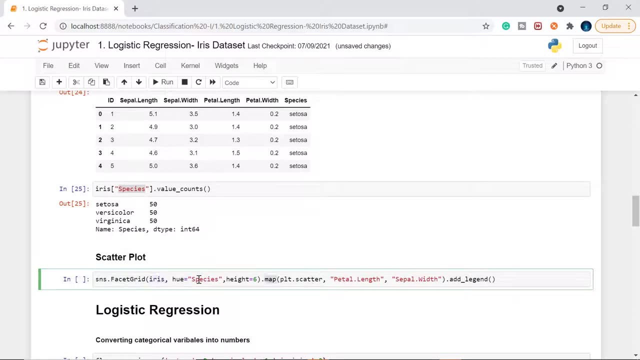 And this is the part of Seaborn library. If you check, we have imported Seaborn as SNS, So I'm using SNS dot facet grid, I raise the data frame and I'm using map function here to plot petal length and sepal width here. 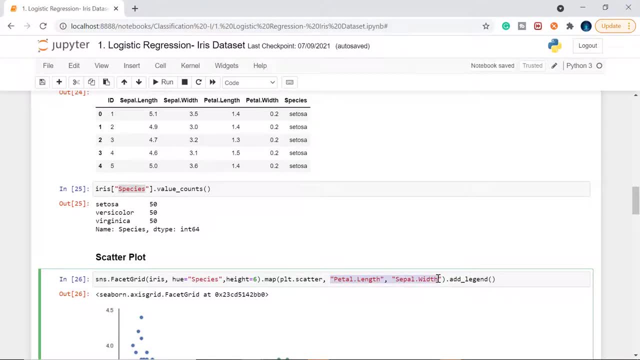 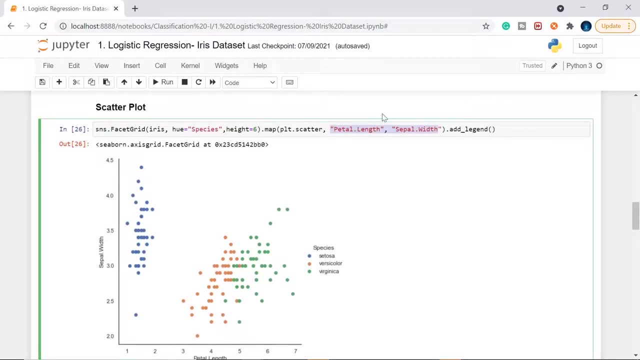 So you can choose whichever columns you want to highlight here. Right, We can visualize, we can plot only two columns, Right So far. now, just for understanding purpose. How does the data look like? I'm plotting this data on petal length and sepal width. 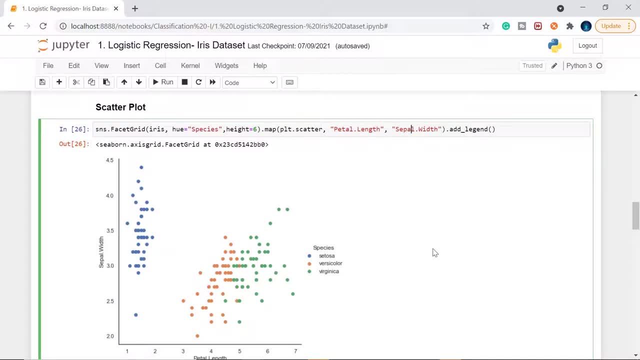 You decide on which you want to plot. OK, so you can see there is a simple classification available. Right Blue ones are separated, The orange and green are a little bit mixed with each other, But these can still be classified with the line. 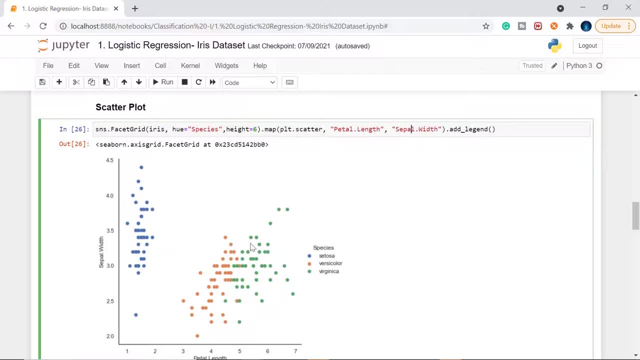 Right, There will be outliers. There will never be a 100 percent accuracy, That's for sure. We'll get 100 percent accuracy for this blue Right. What is this blue set to suffer? set us up? We should get 100 percent accuracy. that I can bet by just looking at the data. 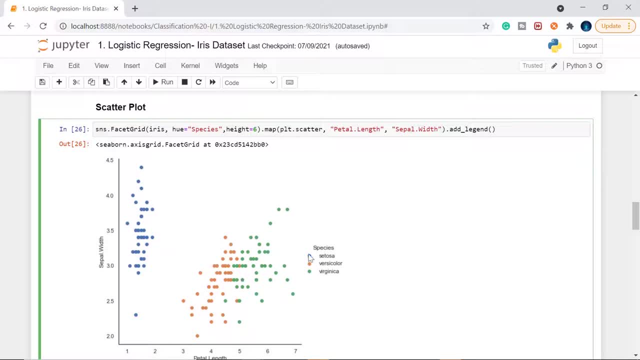 because there is no mixing of blues into the other types, Right. So I can see the legions Blues are the set to suck. Versicolor is orange, Virginica is the green one. There is a bit of a mix here in the versicolor and virginica. 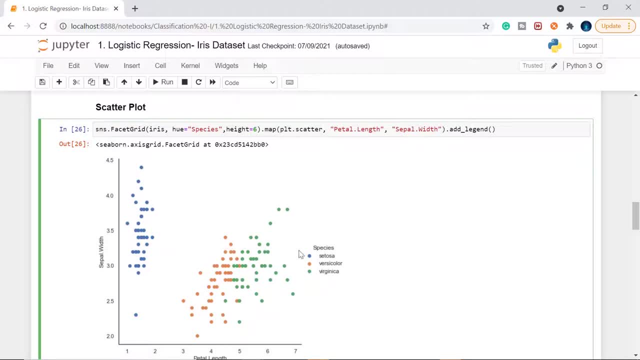 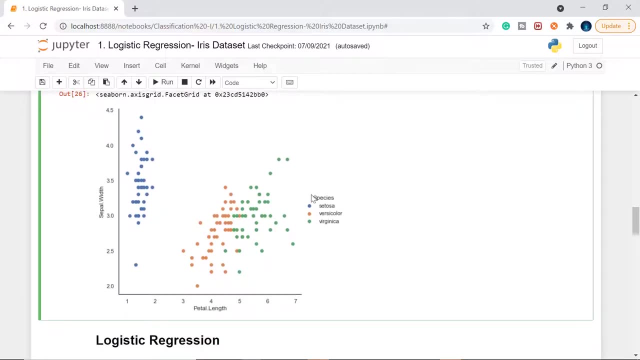 So I may not get to the 100 percent accuracy for versicolor and virginica, But for Setosa I'm I'm sure that we should get. OK, let's see how it goes Now. what next? So machine learning doesn't understand. 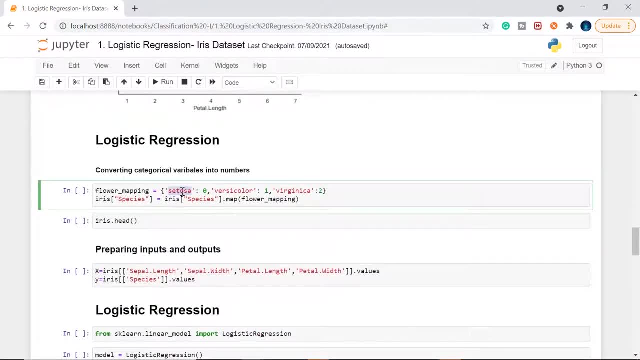 words right? So we will map these words, That is, Setosa versicolor virginica, into the numbers, that is, classes, class zero, class one, class two, and these numbers are nothing but Setosa versicolor virginica. 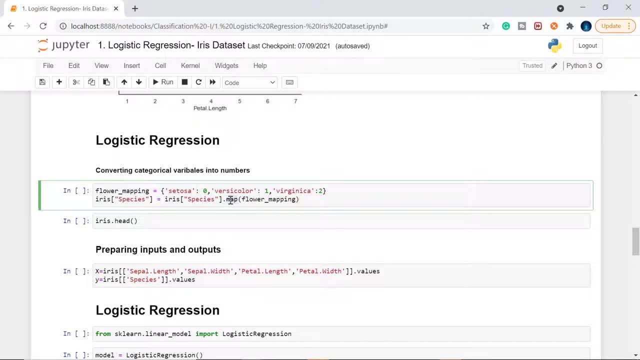 OK, so let's map this by using map function here: Iris species column, map it to floor map. floor mapping is nothing but this dictionary. OK, so mapping is done. So now I have a new column ready with zero one and two. 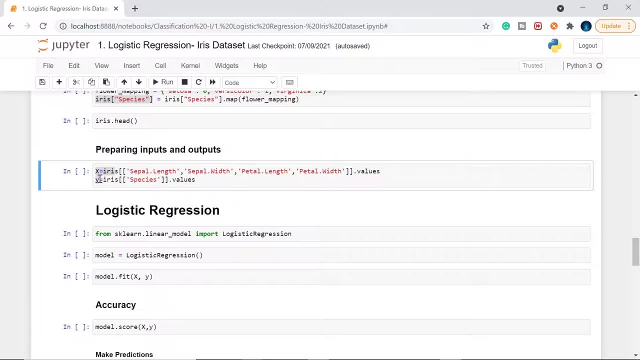 OK, so finally, I have X And Y ready here. So this is the first step that we follow, isn't it? Prepare your X and Y. X is Iris data set, That is data frame. sepal length, sepal width, petal length, petal width values. 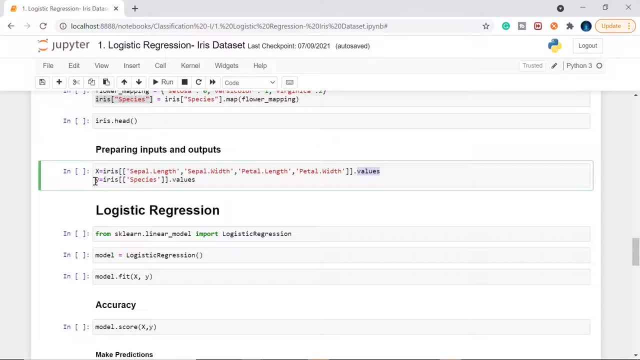 I need values of these four columns. And what is your output? Y is your output And what is the output? The species is the output. right Data frame: species values. OK, so X and Y is prepared. What is the next step? 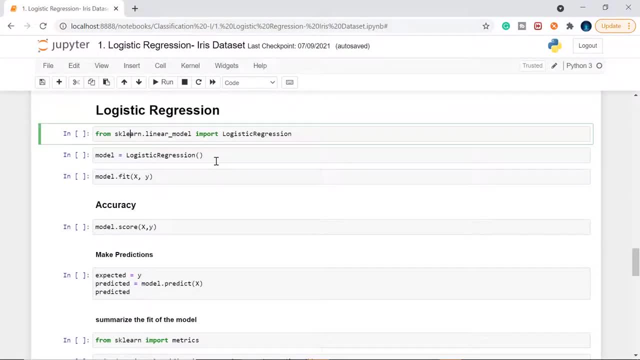 Next step is import your algorithm. So we are using scikit-learn Import logistic regression. It's very simple. Once you import, then initialize right. Model is equal to logistic regression. Open, close rounded packet. So this is the default initialization for now. 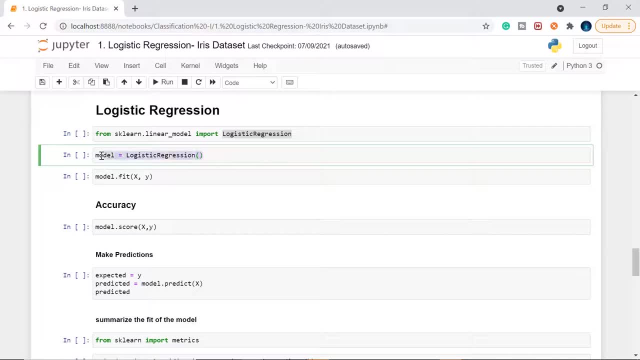 There are also some of the tuning parameters you can pass here, But let's keep that aside for now. We are initializing with the default values. So once you initialize now, we are good to go for the next step, That is, to train the model and find out. 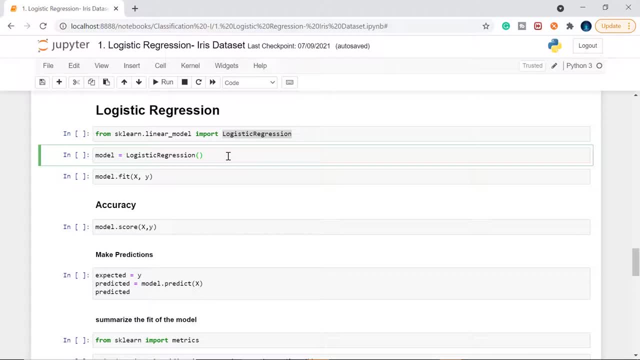 the accuracy or to predict the output for the new values. OK, so to train It's model dot fit. It's that simple. So training happens behind this model dot fit method. Model dot fit function right, Unlike linear regression. when you do model dot fit, it draws a line. 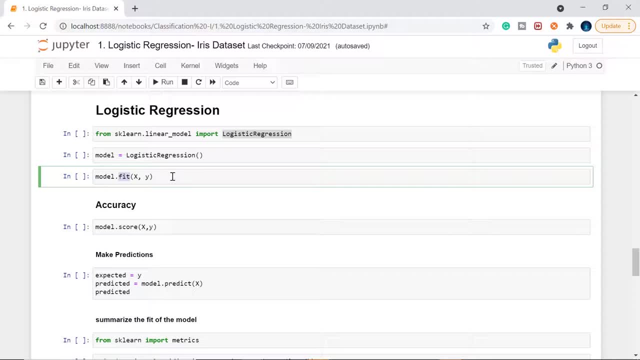 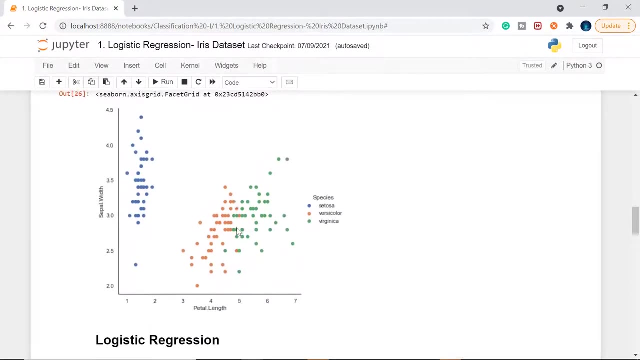 but not to best fit, but to divide the data into two parts, Right. So all that drawing of line and dividing that data into this different part is happening behind this. OK, drawing the best division line right. Division line here And division line may be here, right. 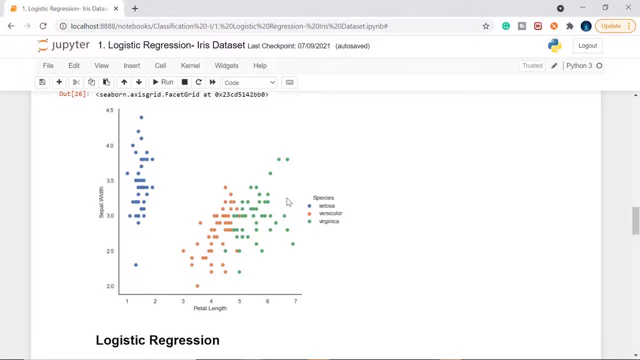 It will be done by machine learning so that when new data point comes, if it falls here, that means it will be a set. So that's how it will be predicting the output for the new data set. Simple, Amazing, right? OK, let me execute this. 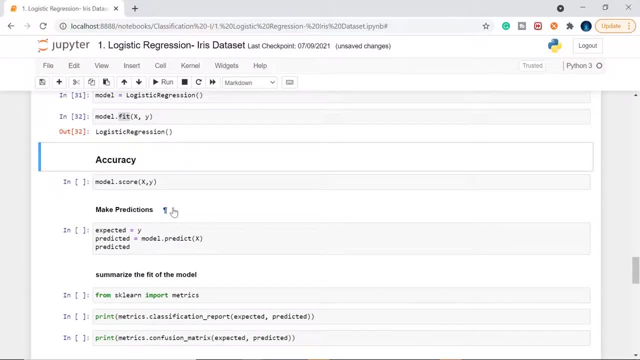 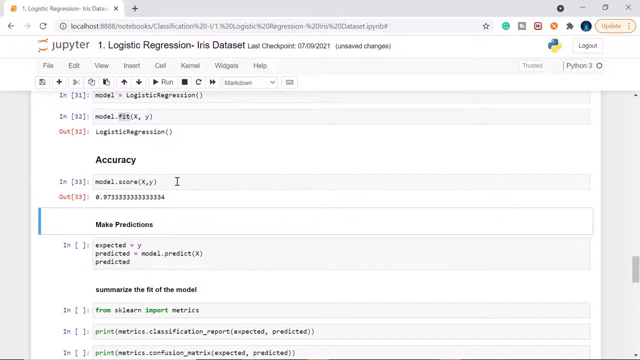 So my model is ready. Let me check the accuracy. And how do we check the accuracy? We have a simple method called score right Model dot score. provide X and Y so that you can see what is the accuracy you have got. 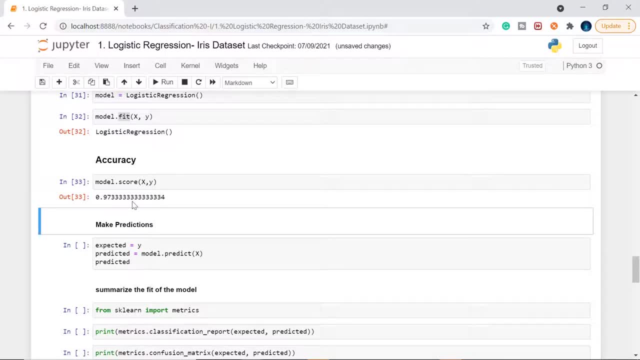 So it's zero, It's 0.9733.. That means we have 97 percent accuracy. OK, though it is not the correct way to measure the accuracy of the model. As we proceed in this series, I will tell you how do we measure the accuracy. 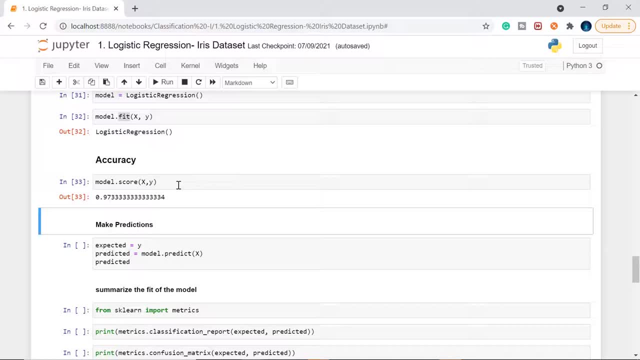 and how can we make our machine learning model better and better and tune our machine learning model so that we get the better accuracy and reduce the noise? OK, but for now it's very simple: right, Model dot, fit, model dot score. 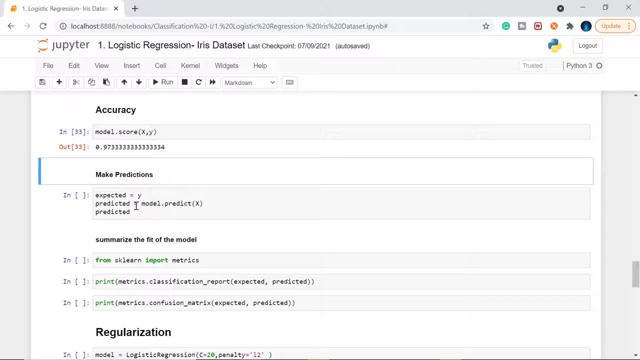 And now let's do the predictions. OK, so to do the prediction here I have a simple method: model dot predict and I'm passing X values. So I'm passing same X values. Let's see what is the prediction I will get for the same input which I have used for the training. 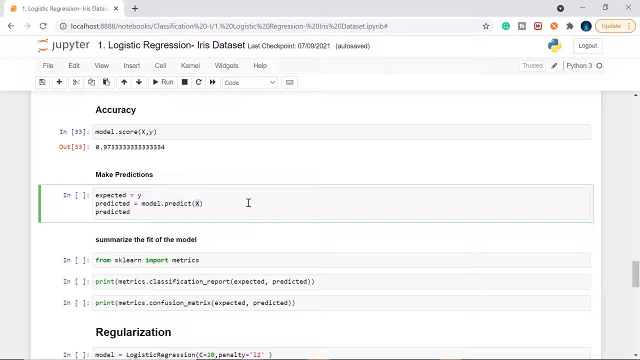 This is the same input, right? I'm not giving any new input here, but the ideal scenario would be provide the new input so that you can get the actual predictions here. But for now I don't have any new input. I'm going to give the same input which I have given during the training. 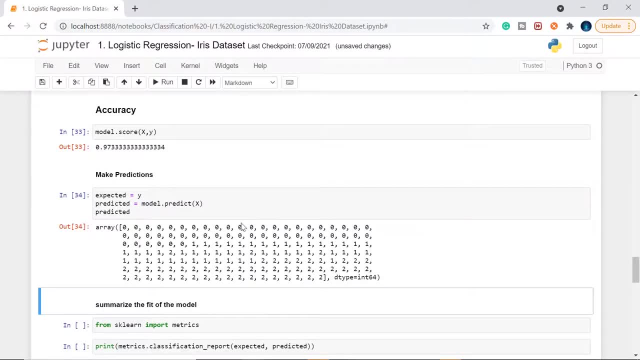 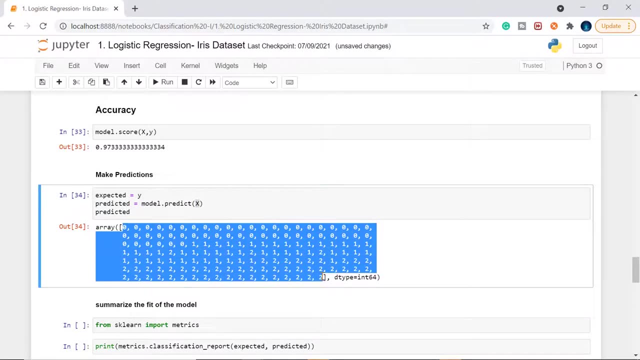 That's again the X. OK, now let's see what is the prediction I'm going to get here. OK, so the predicted is this: for this given input, So for 150 dataset, this is the output I have got. So, if you remember, we have mapped our 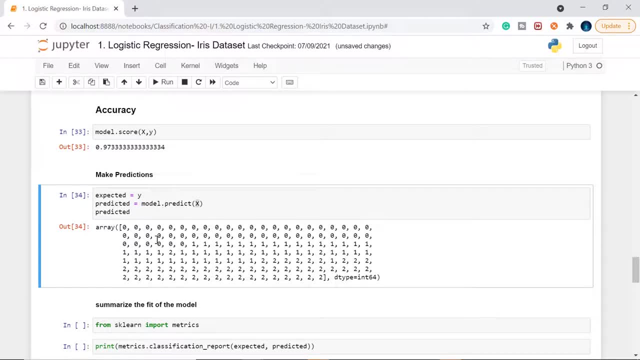 characters, that is, classes, set of our secular version into zeros and ones. That's why I'm getting output in this way. By looking at this, we don't really understand, Right? So what exactly happened here, Whether it is correctly predicted, whether it is not predicted. 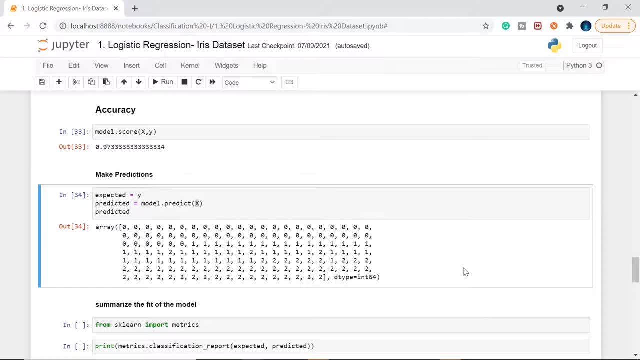 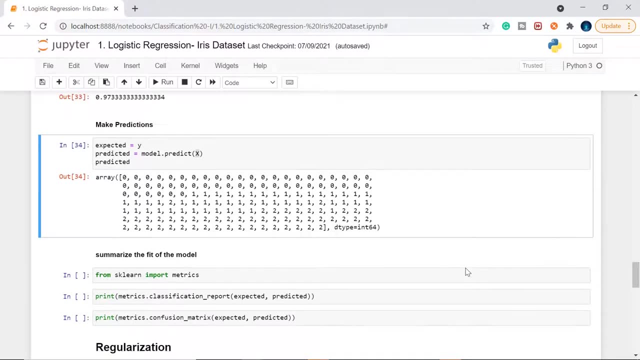 Right. So to understand this output, or a prediction, in a better way, I have something better: matrices. that is called a fusion matrix. It will give us the insights of the predictions. OK, for that I'm using a scale and matrices. OK, so let's import matrix. 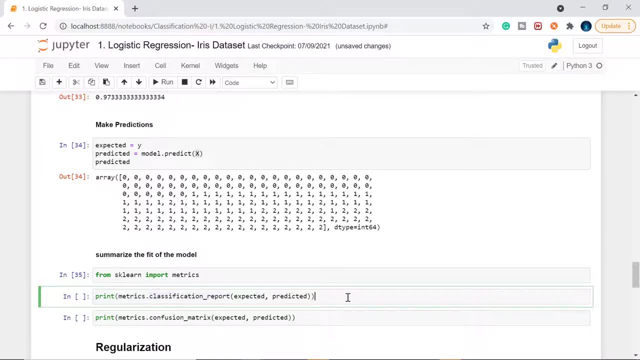 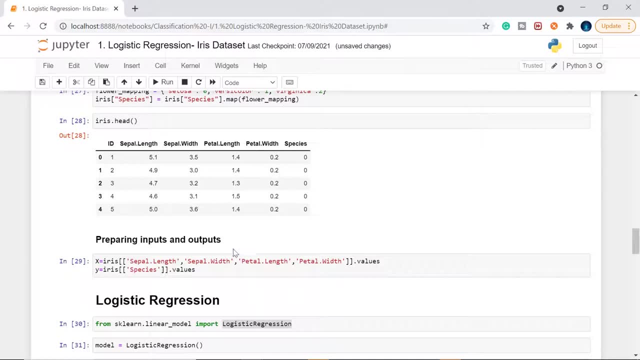 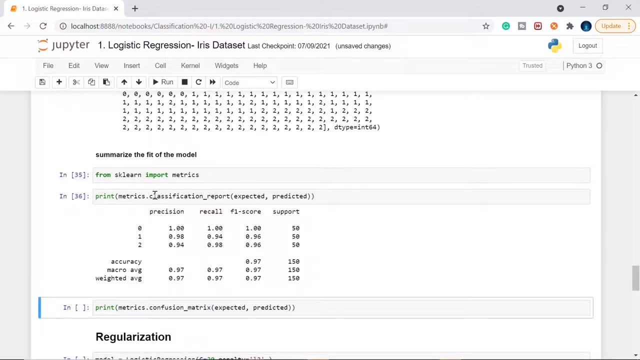 I'm printing the matrix report expected and predicted here. Expected is nothing, but your Y is actual output against the actual output. What is your prediction? That is what I have given your expected and predicted. OK, let's execute this. If you see I have got something called. 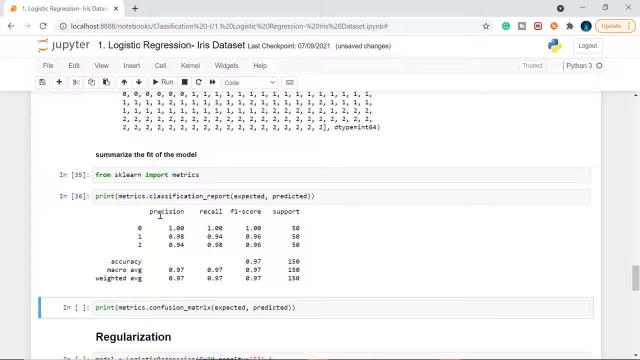 precision recall F1 score Right. So this is a better way to measure your accuracy. OK, Rather than score. you just understand ninety seven percent of accuracy you have got, But you don't really see the insights of the predictions Right? By looking at this you can understand that for zero. 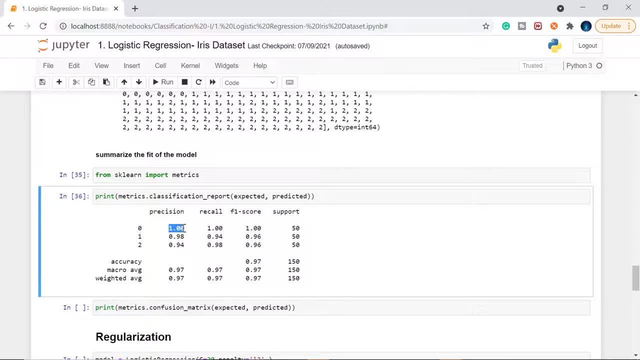 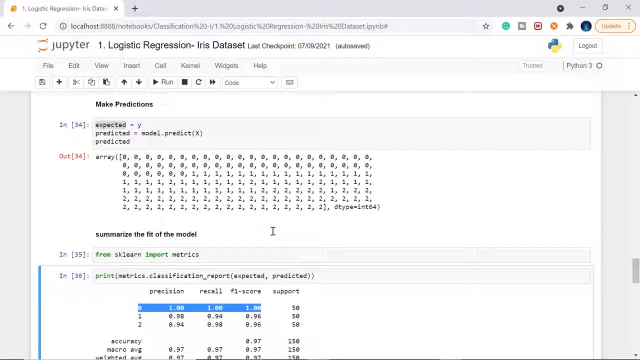 That is for the set of the class. You have precision one, recall one and F1 score one. That means you've got 100 percent accuracy. Do you remember I told you? just by looking at the data It is very easy to classify the set of the flowers. 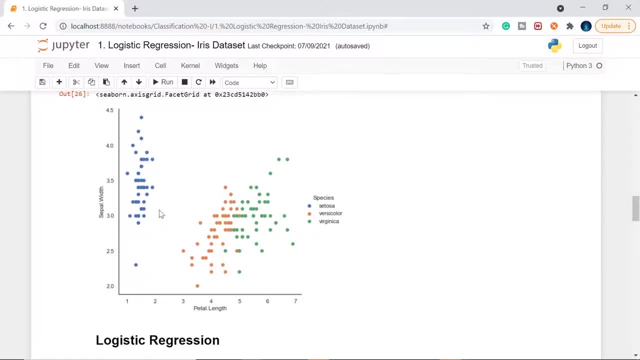 Right. If you draw a line here, it is very easy to classify this Right. There will not be any confusion here at all, but we will have some outliers here will have a confusion here because there is a mix between these two types: Versicolor and Virginica measurements. 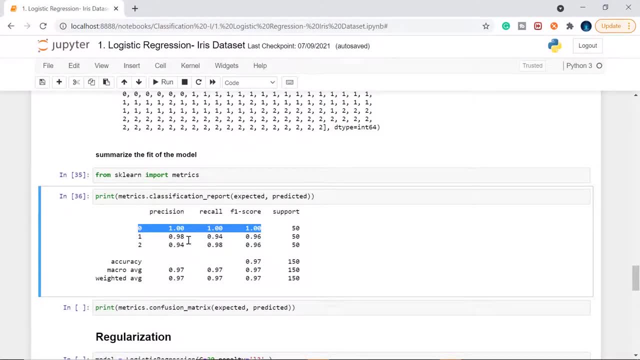 Right, Let's see that. What the precision recall and F1 score sees for the class zero That is set aside is 100 percent. for class one, Versicolor, We have 98 percent precision, Ninety four percent recall and 96 percent F1 score. 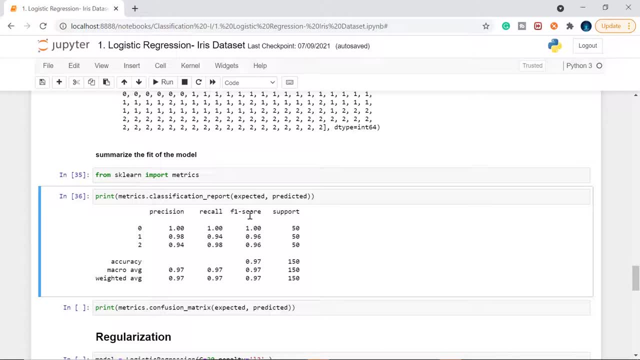 What do you mean by precision, recall, F1 score will understand, maybe in some other videos, But for now you can just say that these are the better ways to calculate the accuracy. All right, Then for second type, for the class to Virginica, we have 94 percent precision, 98 percent recall and 96 percent F1 scores. 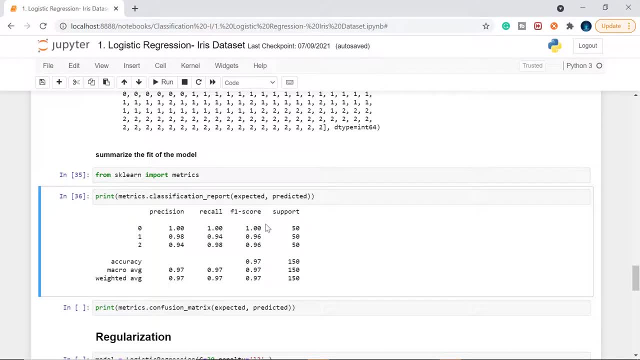 So people will look at the F1 score in general. Right For now, just to understand, You can say that F1 score is the average of precision and recall. So people will always ask you: for what is the F1 score of your model? 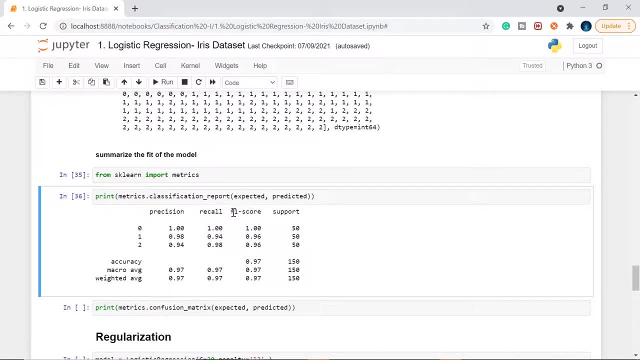 OK, F1 score is a better measure for accuracy. F1 score for set was a type is 100 percent, for Versicolor is 96 and Virginica is 96- again OK, and this F1 score is derived from precision and recall only. 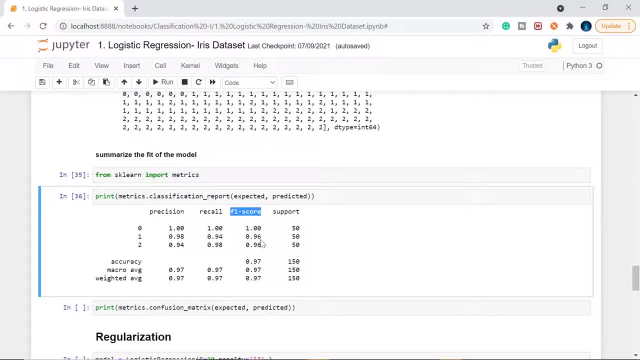 It is always better to give the models accuracy as F1 score. OK, this is what the F1 score stands for: Great, I hope you understood This. we're going to talk about the precision recall F1 score and even the math behind this logistic regression in the other videos. 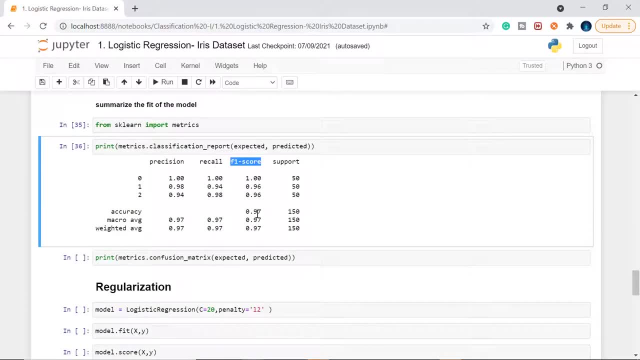 So let's keep that part aside for now. I have one more major to understand the output, the prediction that is called confusion matrix. Once we import matrix, you have classification report and you also have a confusion matrix right. So matrix dot, confusion matrix expected. 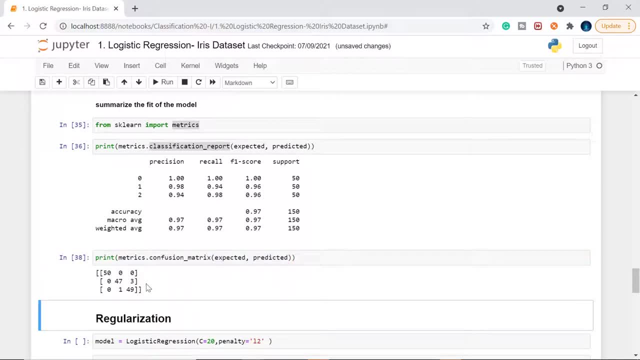 and predicted: OK, let's execute this. What do I get? So I got the matrix here. What I see? 50 0 0. 50 means, if you remember how many data points we had, we had 50 classes each right: Setosa 50, Versicolor 50 and Virginica 50.. 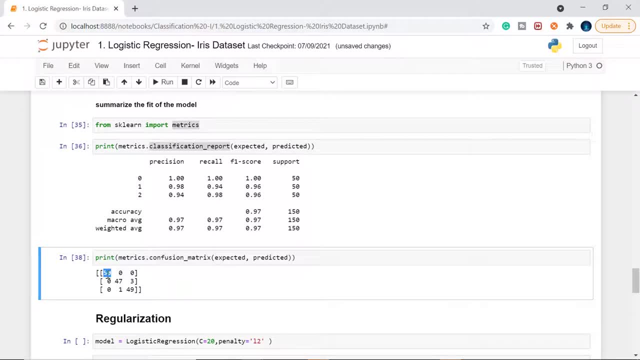 So 50 out of 50 predicted correctly for Setosa. That's what I understand from your 50 0: 0.. No wrong predictions. OK, for Virginica. I can see 47 are correctly classified Right, Whereas three are classified as Virginica. 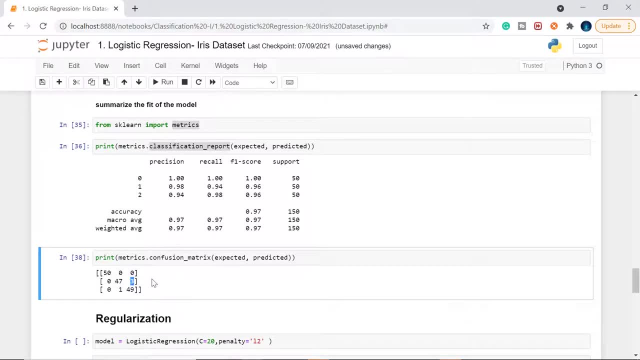 So machine has predicted 47. Correct Versicolor. three Versicolor are classified as Virginica, which is wrong. What about this? If you see here: zero are classified as Setosa, One is classified as Versicolor Right, Whereas 49 are classified as Virginica. 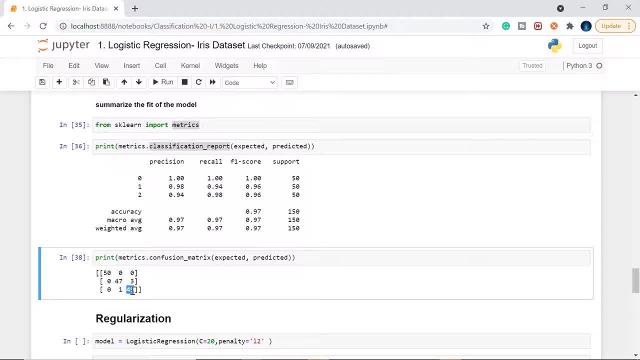 So 49 means there are correct 49 data points classified as Virginica, Only one is wrongly classified. So by looking at this, there is a 100 percent prediction for Setosa and there is a very bad prediction for The second type, that is, Versicolor. and even there is a good prediction for Versicolor.